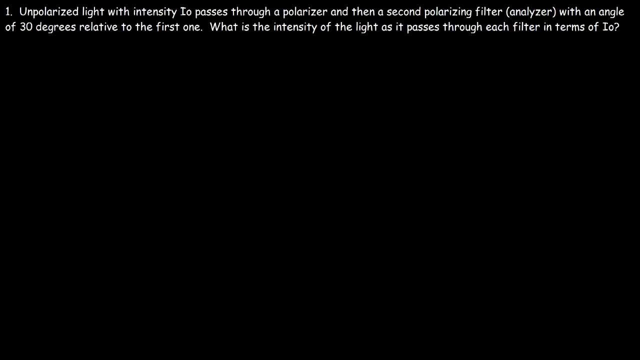 polarizing filter, called the analyzer, with an angle of 30 degrees relative to the first one. What is the intensity of the light as it passes through each filter in terms of IO? So what do you think we need to do? Unpolarized light has light that oscillates in all directions. 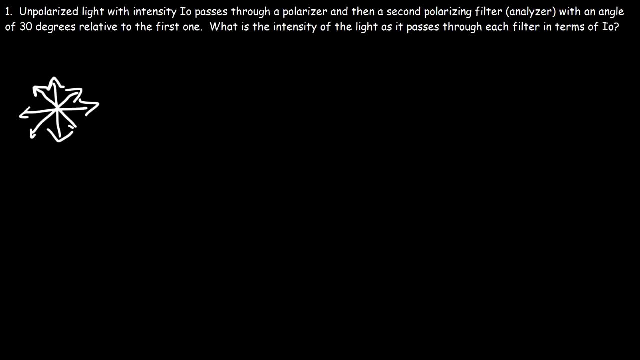 and so we're going to pass it through the first filter and we're going to assume that its axis is vertical, So as light passes through this filter, it's going to be polarized, And so the light will be aligned with this particular. 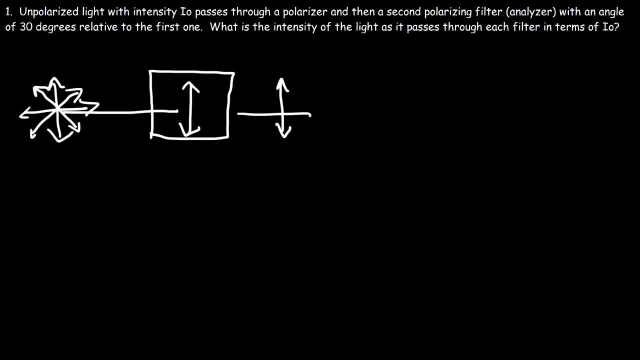 filter, So it's going to be in the same direction as that filter. Now, the initial intensity is IO, So once it passed the first polarizer it's going to lose half of its intensity. So the new intensity is one half of IO. And then it's going to pass through a second filter known. 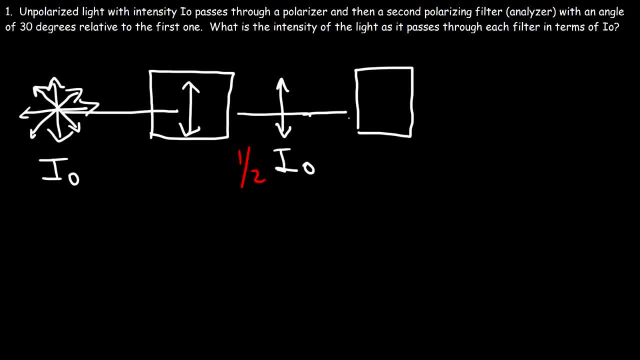 as the analyzer with intensity IO, And then it's going to pass through a second filter known as the analyzer with intensity IO, And this one has an angle of 30 degrees relative to the first one. So if the first one is vertical, this one is going to have an angle of 30 degrees. Now, how can we? 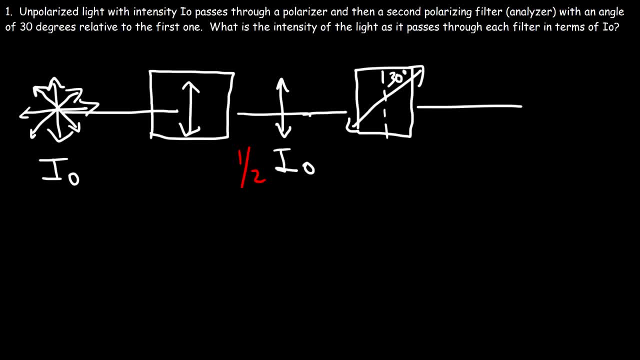 calculate the new intensity. So we could use something known as Malus's Law. Let's call this I1 and this one's going to be I2.. So the intensity that passes through the analyzer, I2, is going to be I1 times cosine squared theta, where theta is the angle between these two filters. 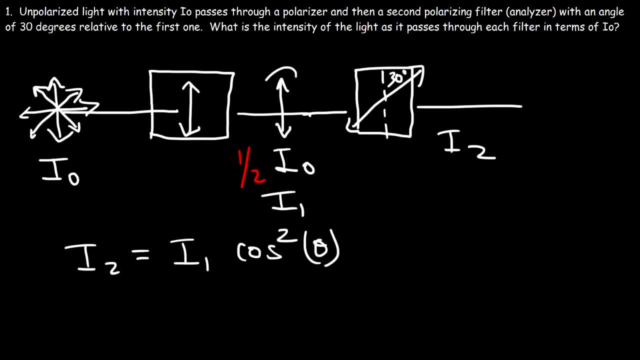 Or you could say: theta is the angle between the light that passes through the filter and the axis of that filter, which is still 30 degrees. So cosine is going to have an angle of 30.. Now, cosine 30 is the square root of 3 over 2, or 0.866.. 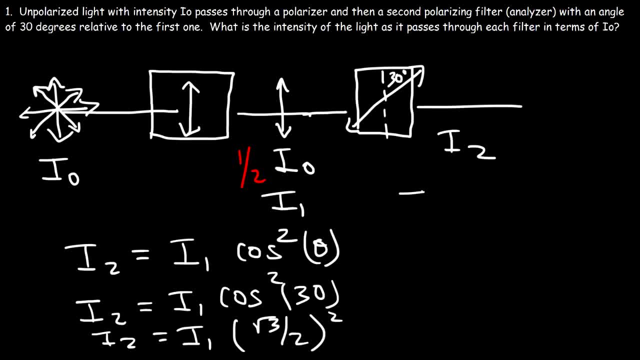 And let's square that. So once we square the square root of 3, that simply becomes 3.. 2 squared is 4.. So I2 is 3 fourths of I1. And we know that I1 is 1 half of the original intensity. 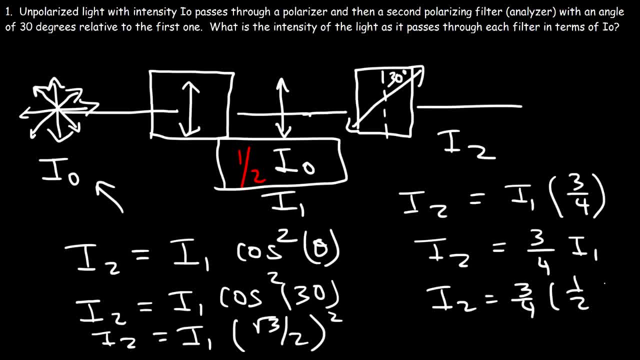 So we can replace I1 with that, And 2 times 4 is 8.. So I2 is going to be 3 eighths of the original intensity, And so this is the answer for the second part of the problem. And this is the answer for the first part of the problem. 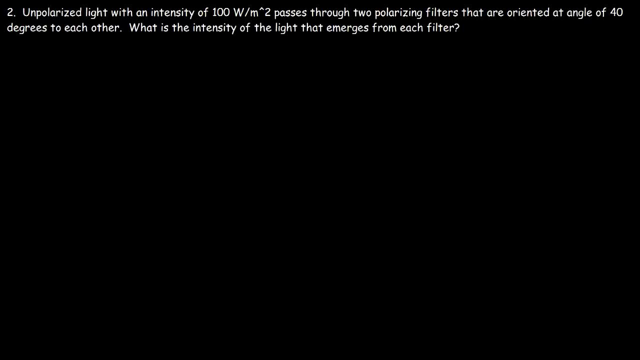 Number 2.. Unpolarized light with an intensity of 100 watts per square meter passes through two polarizing filters that are oriented at an angle of 40 degrees to each other. What is the intensity of the light that emerges from each filter? 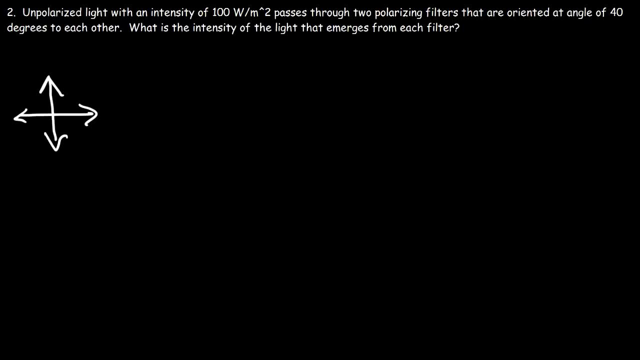 So let's start with unpolarized light, And so it's going to pass through the first filter and then a second filter. Now the first filter. I'm going to say that it's vertical. It really doesn't matter where it is, as long as the second filter is 40 degrees relative to the first one. 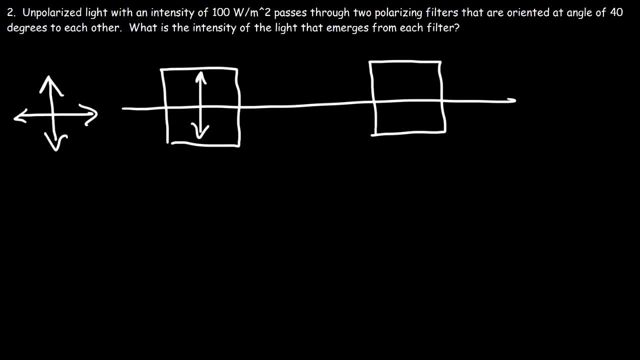 So if this angle is not specified, you can assume that it's vertical And you'll still get the right answer. Now the second filter is 40 degrees relative to the first one. So the first one is, or has, an angle of 0.. 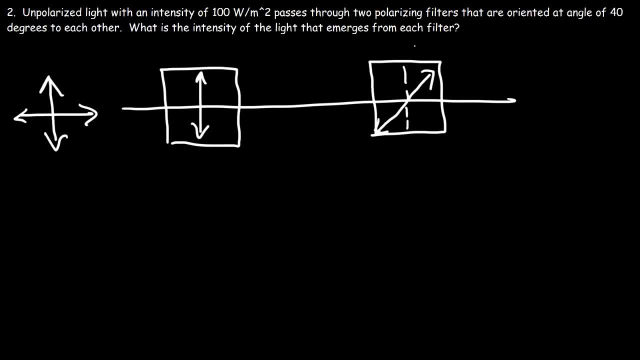 The second one is going to have an angle of 0.. to have an angle of 40 degrees relative to the vertical. So now the intensity of the unpolarized light, Io, is 100.. What is the intensity here? Well, we know that I1, the intensity that passes through the first filter, is going to be half. 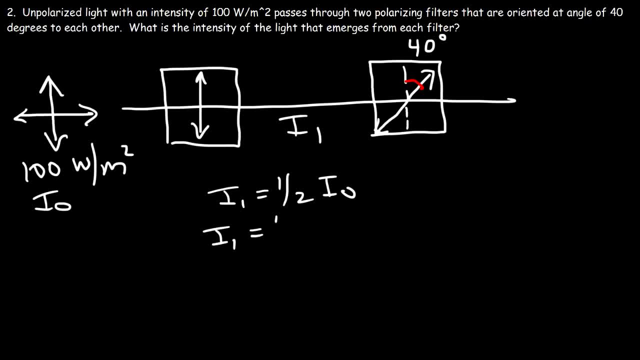 of whatever Io is. So in that case it's going to be one half of 100. And so half of 100 is 50. So it's 50 watts per square meter. So anytime you have unpolarized light passing through the first filter, it doesn't matter. 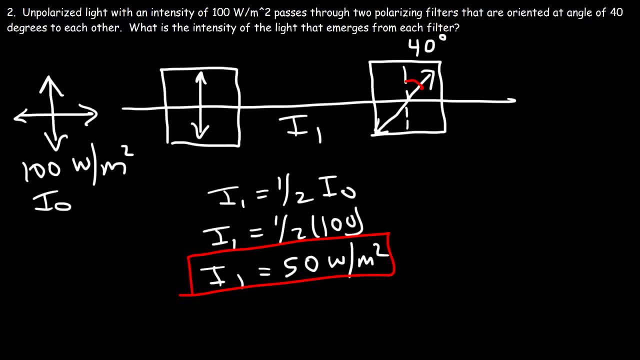 what the angle is. it's always going to be half of the original intensity. Now let's move on to the second part of the problem. Let's calculate Io2.. So, based on Malice's Law, Io2 is going to be I1 times cosine squared of the angle. 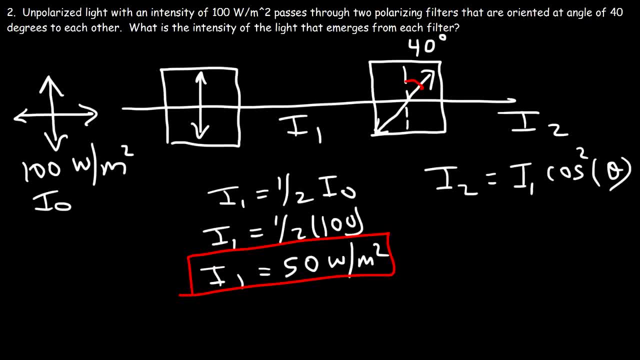 And so the angle is 40 degrees. So we can say that Io2 is I1, I1 is 50, times cosine. squared of 40 degrees, Cosine 40 is like 0.766.. If we square that, that's 0.5868 times 50.. 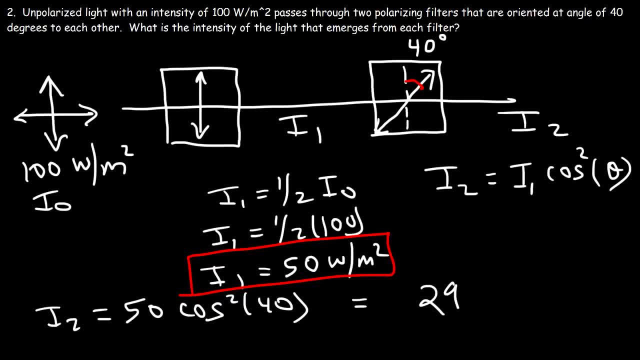 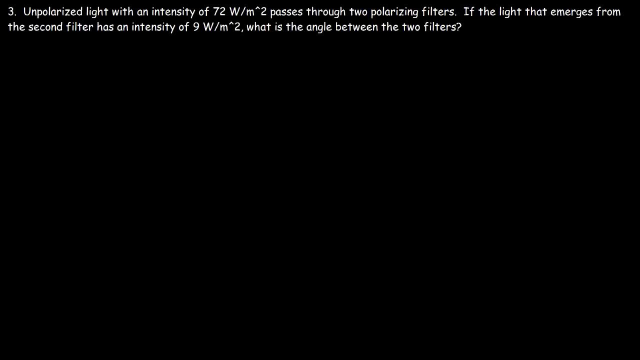 So, then, Io2 is going to be 29.3 watts per square meter. So that is the intensity of the light that is emerging from the second filter, or the analyzer Number three: unpolarized light with an intensity of 72 watts per square meter passes through. 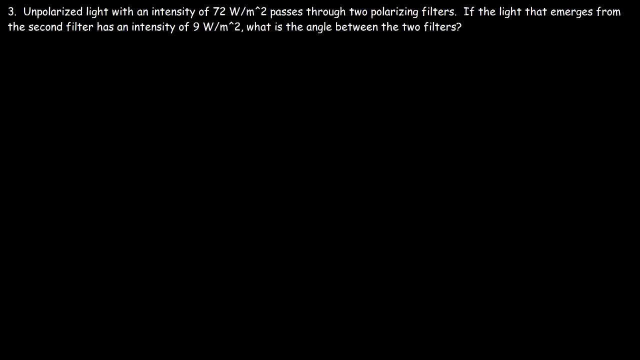 two polarizing filters. If the light that emerges from the second filter has an intensity of nine watts per square meter, What is the angle between the two filters? So let's start with what we know. So the unpolarized light has an intensity of 72 watts per square meter. 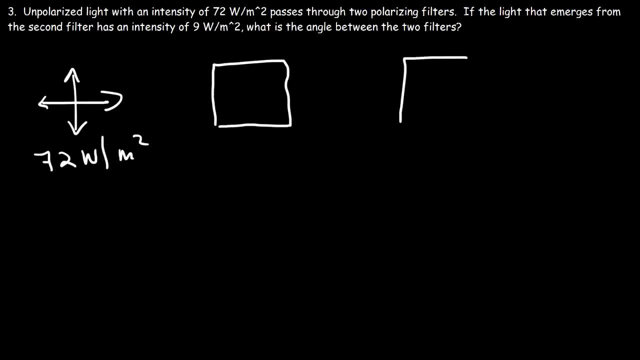 And so here is the first filter and here is the second one. So we're going to say that, once again, this has a vertical axis and the second one has some unknown angle, Unknown angle which we'll call theta. How can we calculate the angle between the two filters? 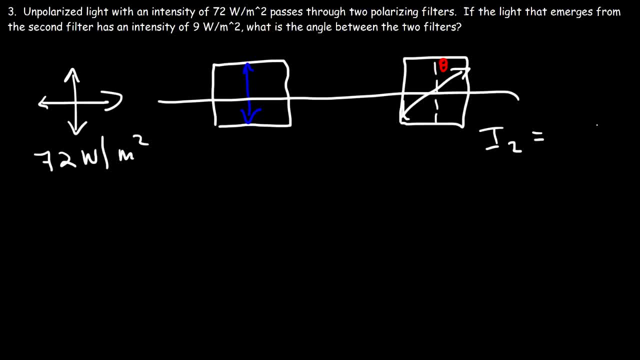 We know the second intensity: It's equal to nine watts per square meter. So what should we do? First, we need to come up with an equation that describes I2 and Io. We know that I1, the intensity after the light passes through the first filter. it's one. 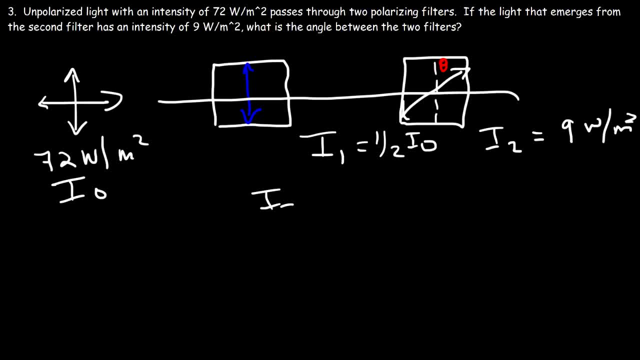 half of I0.. And I2 is equal to I1 times cosine squared, based on Malus' law. So let's replace I1 with one half Io, So we can say that I2 is one half of Io times cosine squared theta. 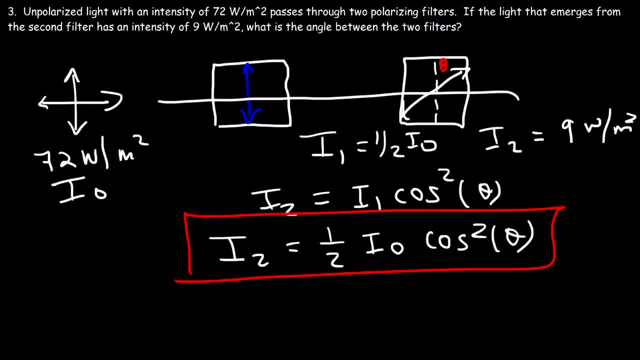 And so this is the equation that we need in order to calculate. So let's go ahead and do that. So we know that I2 is nine and Io is 72. So half of 72 is 36.. Now I'm running out of space, so let me just get rid of this stuff. 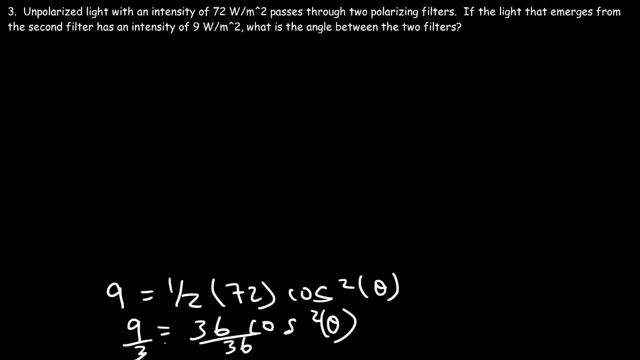 So now let's divide both sides by 36.. 36 divided by nine is four. so nine over 36 is one fourth, And so that's equal to cosine squared theta. Now let's take the square root of both sides. The square root of one is one and the square root of four is two. 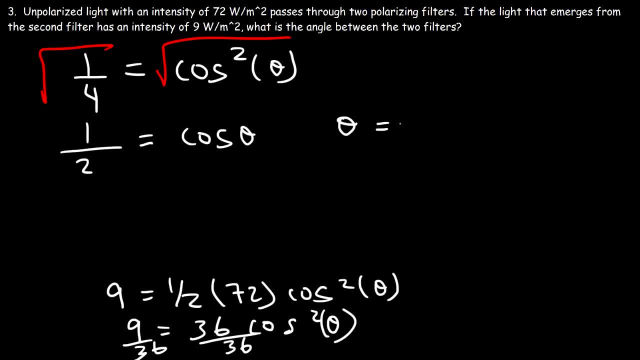 So one half is equal to cosine theta. Theta is going to be the arc cosine or the inverse cosine of a half. So at this point you can just type that in your calculator. Make sure that it's in degree mode. So theta is 60 degrees and that's the answer. 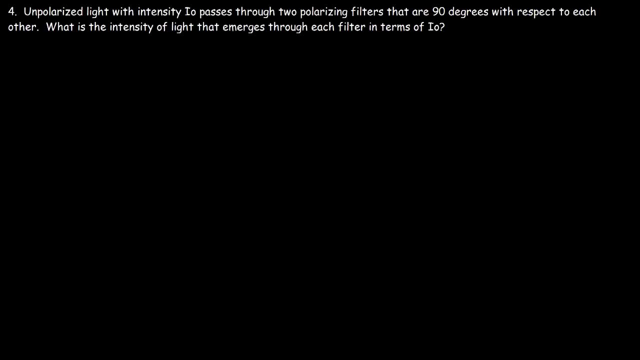 So that's the angle between the two filters. Number four: unpolarized light with intensity Io passes through two polarizing filters that are 90 degrees with respect to each other. What is the intensity of light that emerges through each filter in terms of Io? 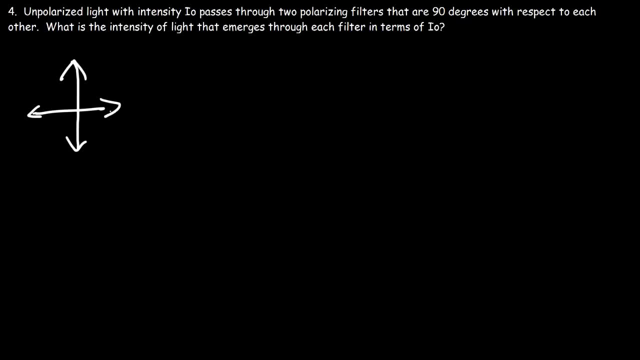 Let's find out, Okay. So let's start with our unpolarized light and let's pass it through two filters Now. the first one- we're going to say that it's vertical, And the second one is 90 degrees with respect to the first one. 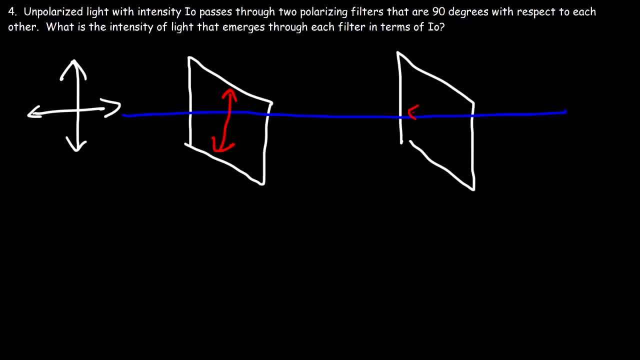 So the second one has to be horizontal. Okay, So the light that passes through the first filter, it's going to be in the direction of the first filter, It's going to be parallel to it. So if this has an intensity of Io, the second one is going to be half of Io. 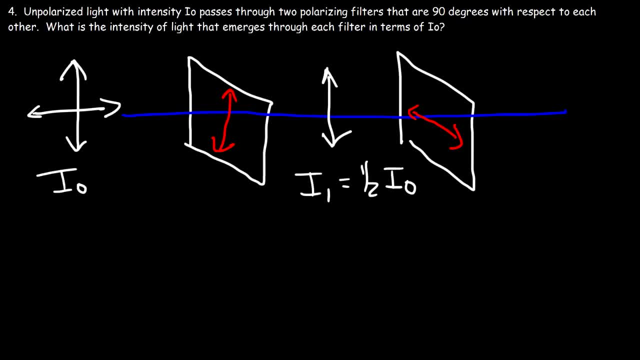 Now what about the third one? So what is I2?? So I2 is equal to I1 times cosine squared. Okay, So I2 is equal to I1 times theta squared. Okay, So I2 is equal to I1 times theta squared. 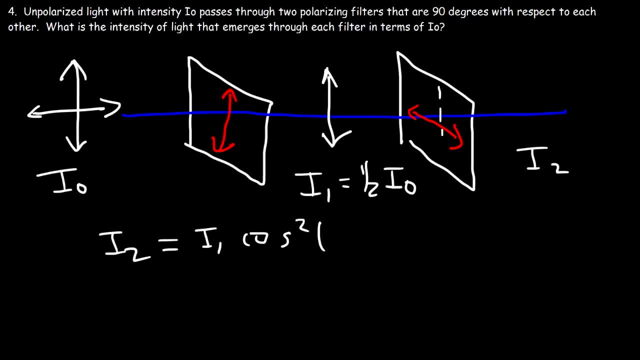 Now the angle is 90 degrees with respect to the first one, And so this angle right here is 90 degrees, So we can draw a box, And so theta is 90.. And cosine 90 is 0.. So therefore, I2 will be equal to 0. 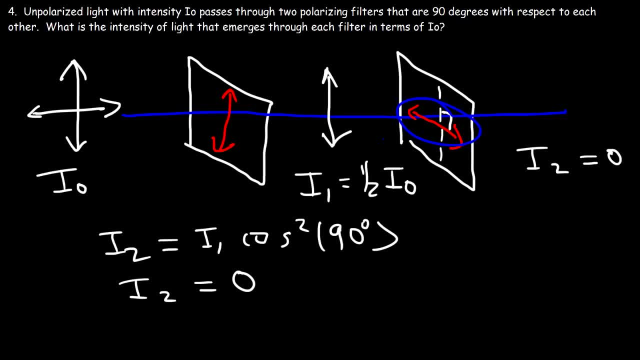 So whenever the axis of the polarization changes, Okay, Of the polarizing filter, if it's 90 degrees with respect to the light that's coming in, then no light will be transmitted. And so these are the answers. So the first answer, the intensity, is one half of the original intensity after passing. 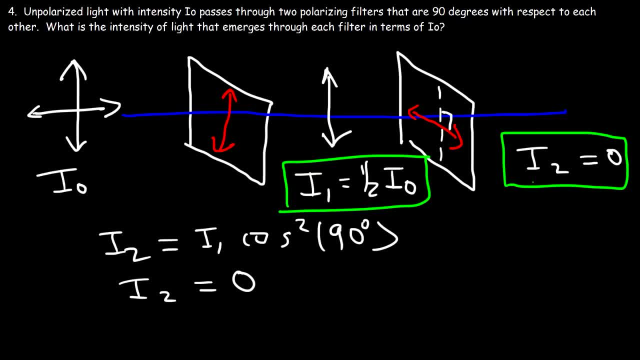 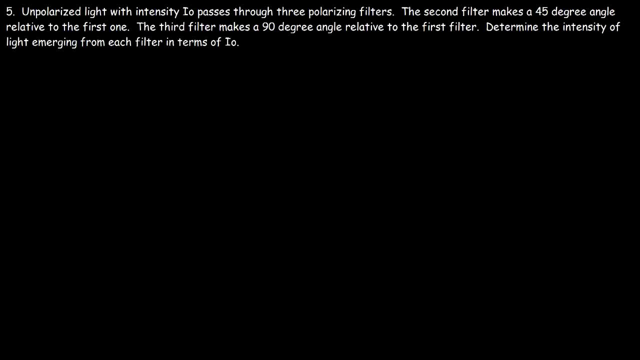 through the first filter, as always, But through the second filter it's going to be 0. Number five: Unpolarized light with intensity Io Passes through three polarizing filters, So let's draw a picture. This is going to be the first one. 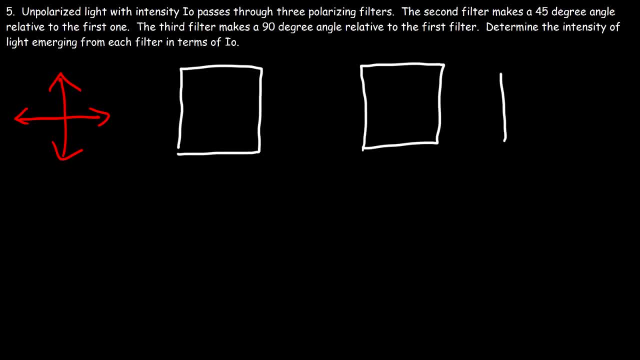 This is going to be the second one, and here is the third one. Now, the first filter we're going to say has an angle of 90. I mean that angle of 90, but let's just say that it's a vertical. and The second filter makes a 45 degree angle relative to the first one. 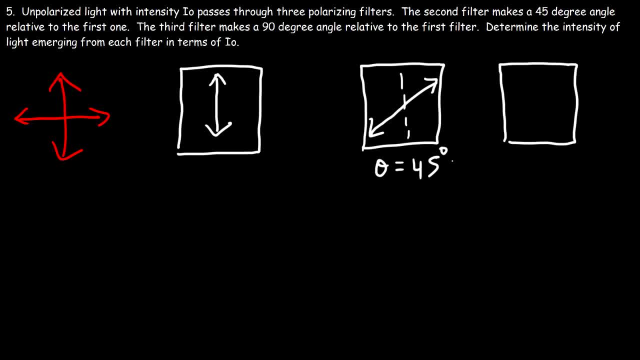 So this is 45 degrees relative to the vertical, and the third filter makes a 90 degree angle relative to the first one, So theta will be 90 with respect to the vertical. Determine the Intensity of light emerging from each filter in terms of IO. So this is going to be IO I one is going to be one half of. 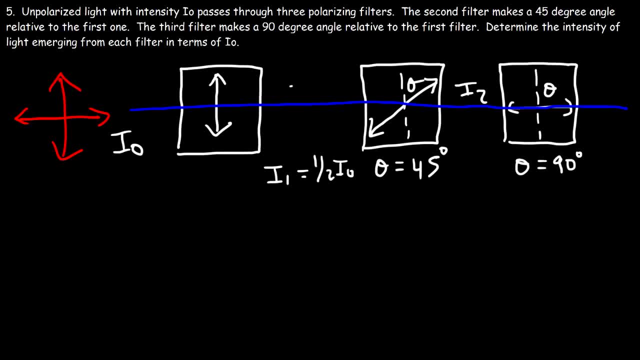 IO. and then here we have I two and I three. So what's I two in terms of I one? well, based on Malice's law, I two is going to be I one times cosine squared theta. So I one is one half of IO and the angle is 45 degrees. 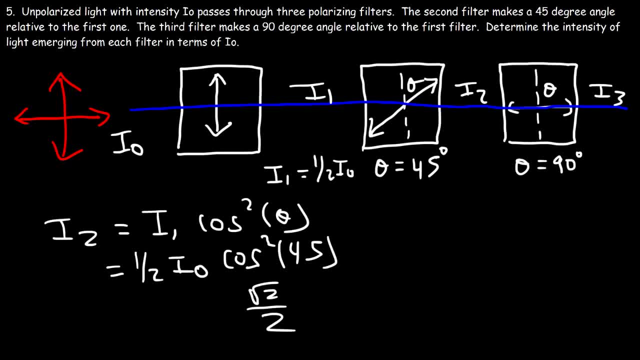 Now, cosine 45 is equal to the square root of 2 divided by 2, and we need to square it. So the square root of 2 squared is 2 and 2 squared is 4, so we could cancel these two and So it's 1: 4th of I: 0. 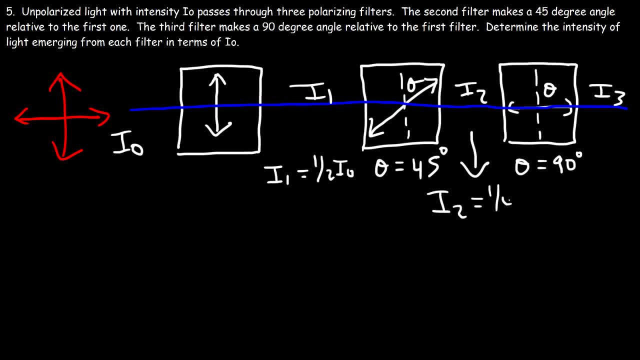 So let's write this answer here: I 2 is going to be 1, 4th of I 0, and so this is the first answer that we're looking for and This is the second answer. So now let's draw the light that passes through. 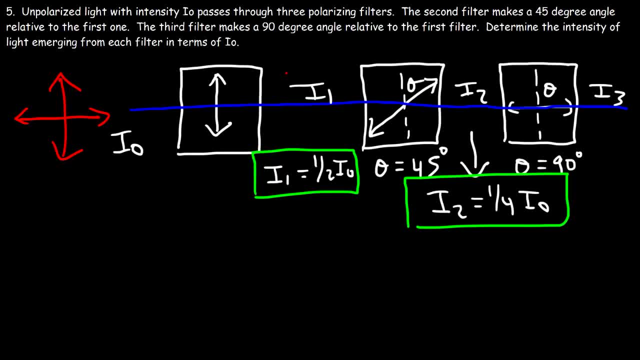 Each filter. So the length that passes through the first filter will be in the direction of the first filter. The light that passes through the second filter will be in a direction of the second filter, but with every reduced intensity. So we should draw it like smaller, Maybe like that, and then the third one will be in a direction of this one, but even smaller. 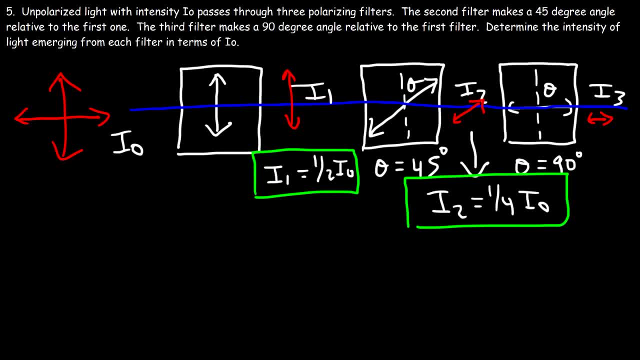 So the light that passes is through the filter will always have the same direction as the filter itself. Now let's calculate I3 in terms of I2 first. So once again we can use Mallet's Law. Now I2, we know it's 1 fourth of I0. 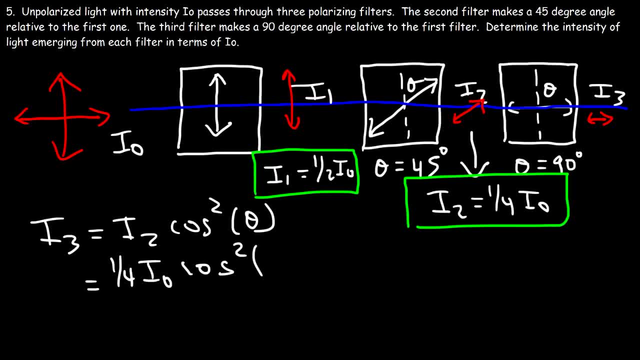 Now, what is the angle that we should use here? Is it 90 degrees or is it something else? The angle is not 90 degrees. Technically speaking, the angle is between the axis of the filter and the axis of the light that passes through the filter. 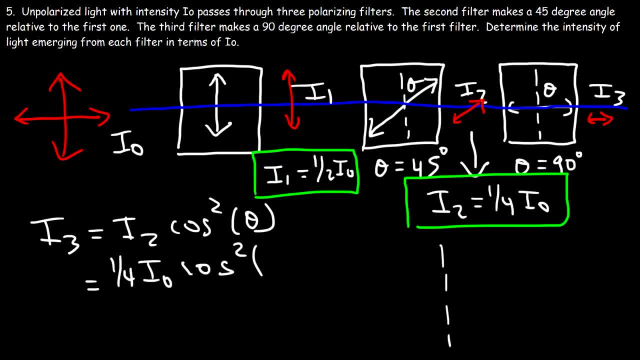 So let's draw a picture. So the filter is here. It's 90 degrees with respect to the vertical. Now the light that passes through the filter is 90 degrees. Now the light that passes through the filter is 90 degrees. Now the light that passes through the filter is at a 45 degree angle relative to the vertical. 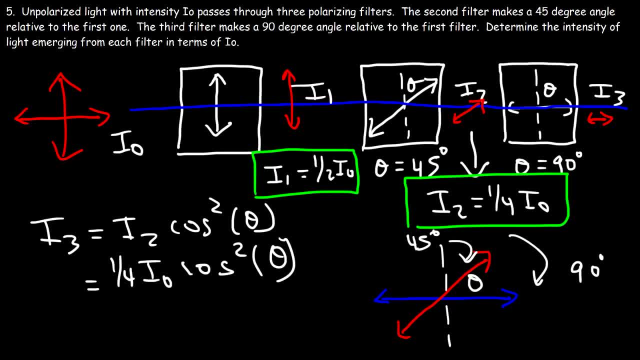 So this angle that we need to use in this equation is really the difference between these two angles. So it's 90 minus 45, which, for this example, is 45. So this is the angle that we're looking for, the angle between the filter and the. 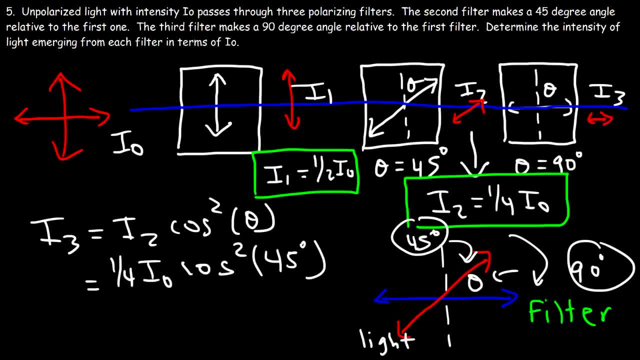 angle between the polarized light. So let's go ahead and finish this problem. So cosine 45, that's the square root of 2 over 2. And if you square it it's going to be 1 half. So 1 fourth times a half is 1 eighth. 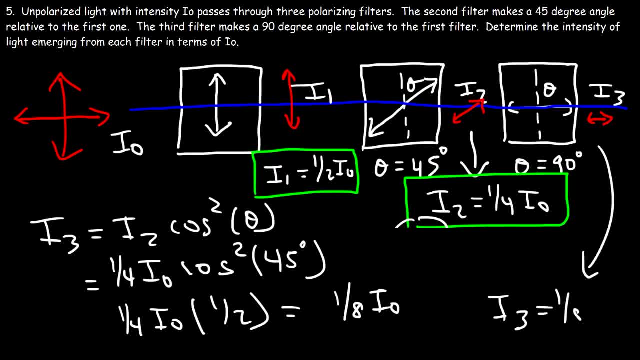 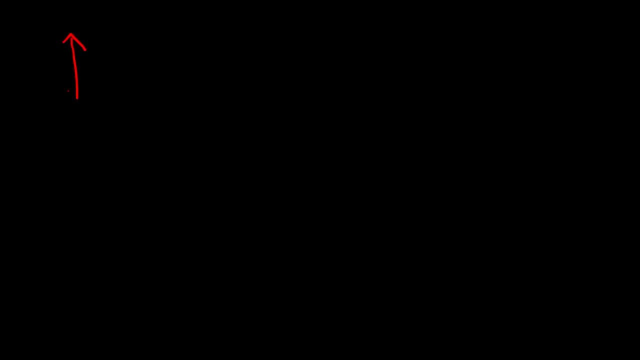 So I3 is going to be 1 eighth of the original, And so this is the answer we're looking for. So these are the three answers. Now I'd like to take a moment to review the significance of the last two problems. So in problem number four we had two filters. 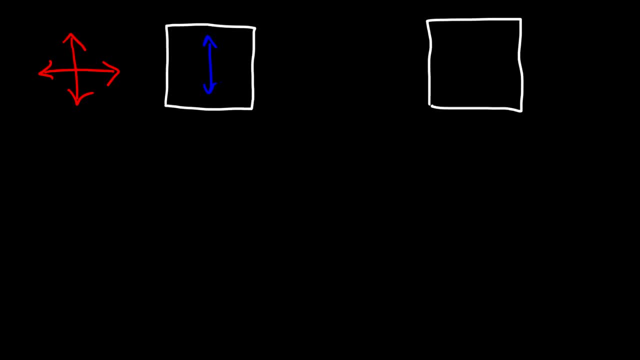 The first filter had a vertical axis and the second one had a horizontal axis, And we saw that the intensity of light Emerging from the second filter was equal to zero, Because cosine 90 is zero. Now, in the fifth problem, what we have done is basically add a filter between these two. 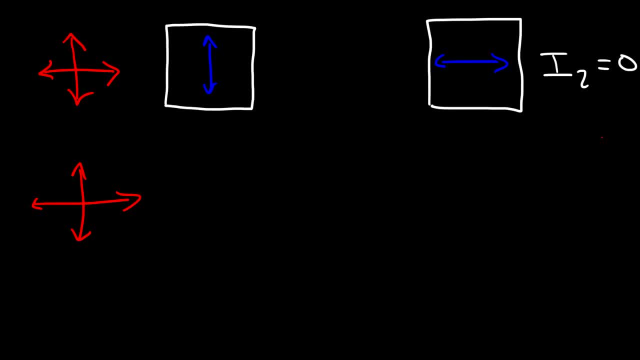 filters. So notice what happens to the final intensity if we add a third filter in between. So we still have these two intensities, I mean these two filters rather. But the third filter had an axis that was 45 degrees relative to the vertical. 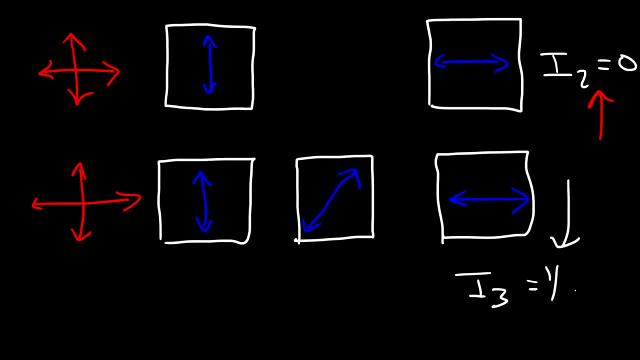 And so this intensity I3, we saw that it was 1 eighth of I0. So by adding a third filter in between these two filters that are 90 degrees apart from each other, we were able to increase the final intensity from zero to a higher value. 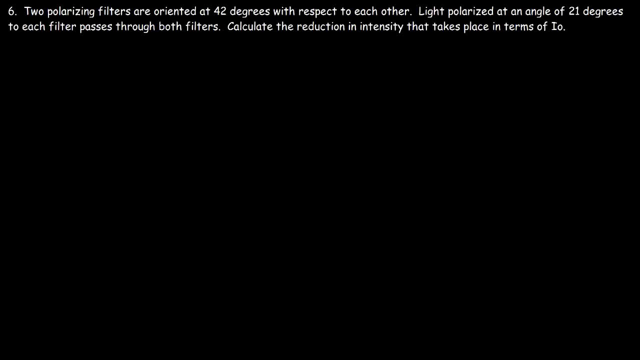 Number six. two polarizing filters are oriented at 42 degrees with respect to each other. Light polarized at an angle of 21 degrees to each filter passes through both filters. Calculate the reduction in intensity that takes place in terms of I0. 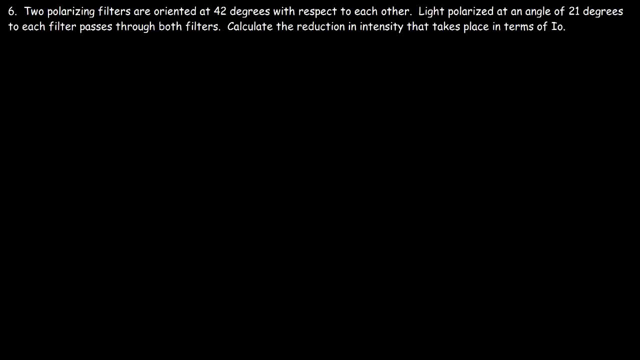 Go ahead and try this problem. So what do you think we need to do? Let's say that the first filter is vertical and the second one is going to be at an angle of 42 degrees relative to the vertical line. The first thing we need to do is understand the problem. 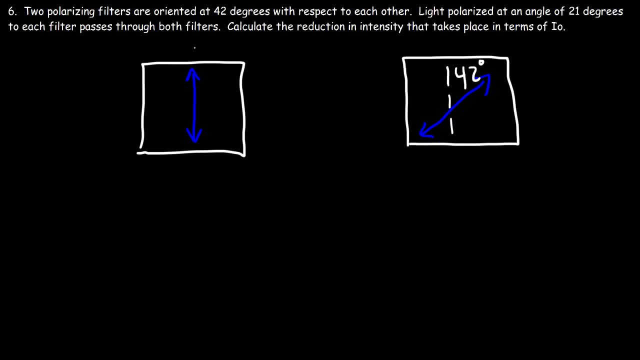 Once we can do that, then we can find the answer. So that's the first thing we know. The two filters are oriented at 42 degrees with respect to each other. So what do you think we need to do? Let's say that the first filter is vertical and the second one is at an angle of 42 degrees. 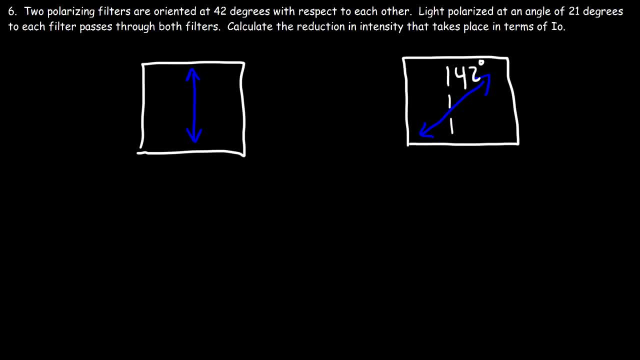 relative to the vertical line. Now, we don't have unpolarized light at the beginning, Rather, the light is already polarized, And so we need to be careful with that statement. And it's polarized at an angle of 21 degrees to each filter. 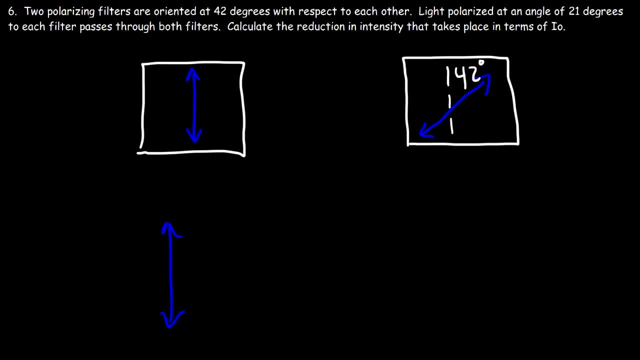 So if the first filter is at an angle of zero and let's say the second filter is at an angle of 42,, then the light has to be at an angle of 21.. Because if this is zero and this is 21,, then the light is already polarized. So we need to be careful with that statement. Let's say that the second filter is at an angle of 42. Then the light has to be at an angle of 21. Then the light has to be at an angle of 41 and that's 42.. 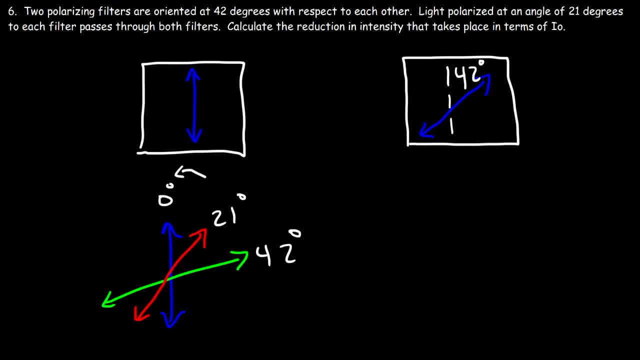 The light is 21 degrees from both filters, So this angle is 21 and this angle- the difference between 42 and 21- is still 21.. So the light that enters this filter is at a 21 degree angle relative to the vertical. 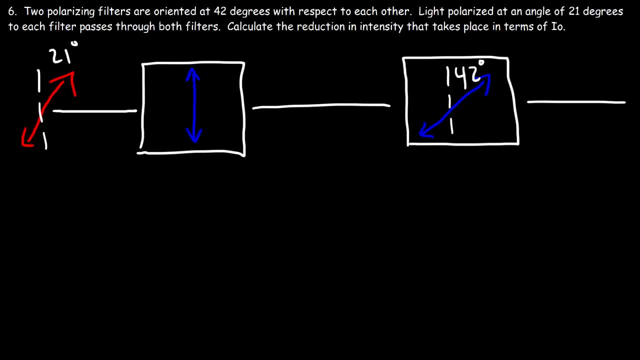 Now, the light that leaves this filter will be in the same direction as that filter, And the light that leaves this filter will be in the same direction as that filter, And so it's important to understand that concept. So let's call this I0, and this is going to be I1 and that's I2.. 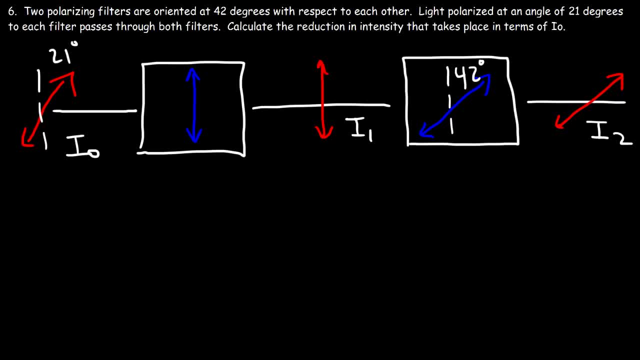 So let's calculate I1 and I2 in terms of I2.. I0 first, and then we can calculate the reduction in intensity later. So we can't say that I1 is half of I0.. We cannot do this, And why is that? 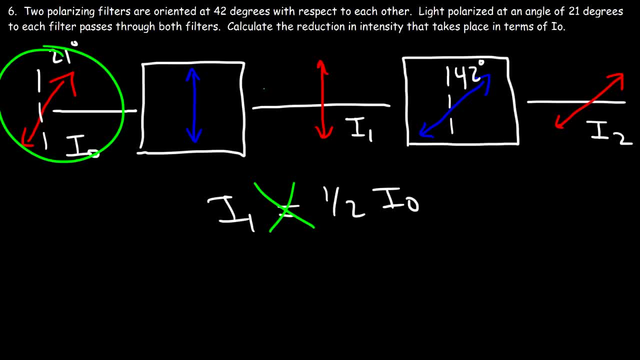 This is only true if we have unpolarized light becoming polarized. but we don't have that. This light is already polarized, So therefore we need to use Malice's law to get I1.. So I1 is equal to I0 times cosine squared theta, and so this is at an angle of 0 degrees. 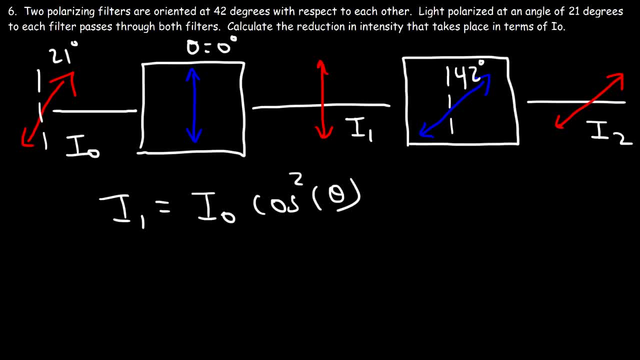 and this is 21 with respect to the vertical. So the difference in angles is 21 degrees. So I1 is equal to I0 times cosine, 21 degrees squared, And so we can say that I1 is 0.8716 of I0, so I'm just going to write that here. 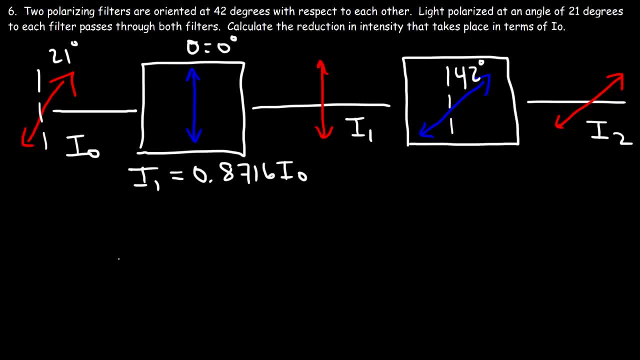 Now let's move on to the second part. Let's go from I1 to I2.. So I2 is equal to I1 times cosine squared theta. Now I1 is equal to this thing, so we could replace I1 with 0.8716, I0, and the angle between: 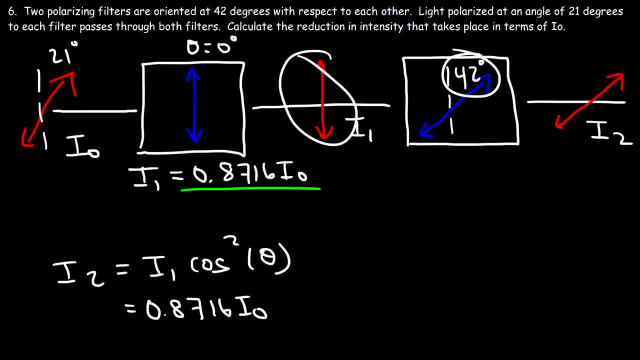 the plane, polarized light and the filter. so this is at an angle of 0 degrees relative to the vertical and this is 42. So the difference is 42. So we're going to have cosine squared of 42 degrees. Cosine 42 is 0.7431.. 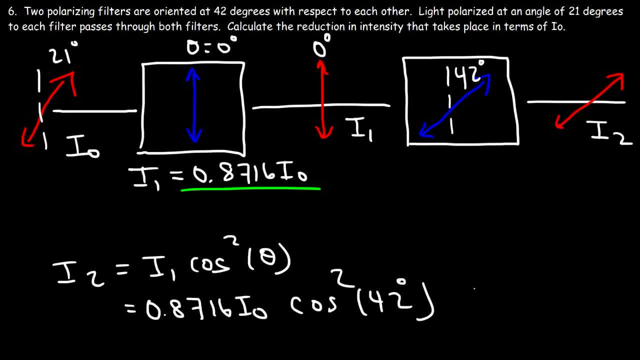 If you square that, that's 0.55226 times 0.8716.. And so we could say that I2 is equal to 0.4814, if you round it relative to I0.. But we're not done yet. 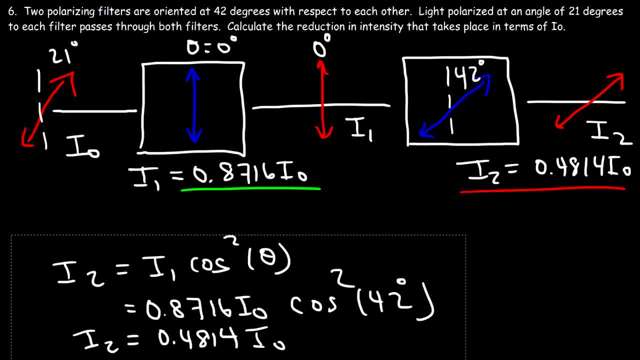 We still need to calculate the reduction in intensity. So what this equation is telling us is that I1 is 87.16% of I0.. Now, I0 was the original intensity. it represented 100%. So if you go from 100% to 87.16%, 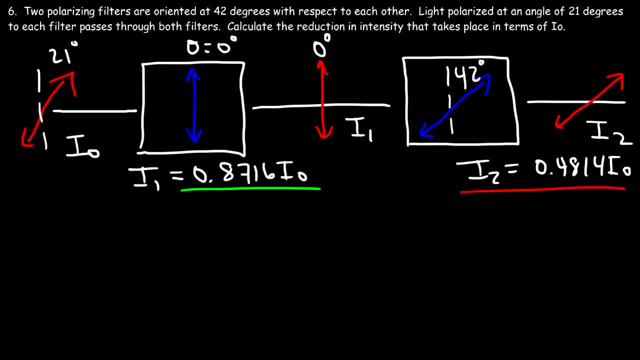 It's a reduction. It's a reduction of 12.84.. So to calculate the reduction, just take 1 and subtract it by 0.8716.. And so the reduction in intensity. you could say it's 12.84%. 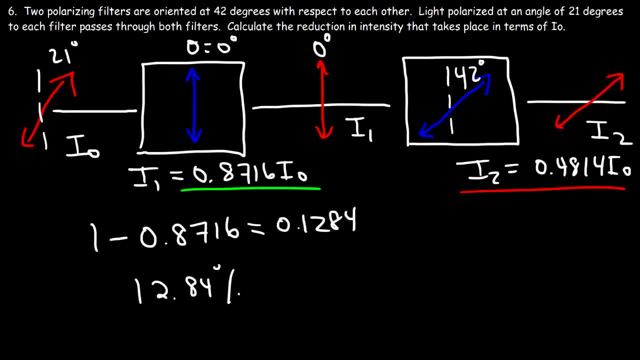 This is equal to 0.1284.. So if you multiply it by 100%, that's 12.84%. So that's the reduction passing through the first filter. Now for the second filter. It's going to be 1 minus 0.4814. 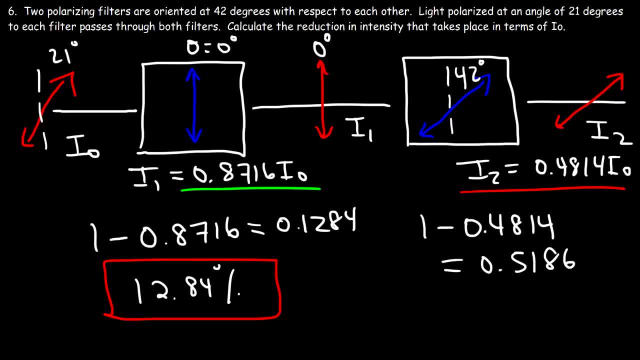 And so that's 0.5186.. And then if you multiply that by 100, then the intensity was reduced by 51.86% relative to its original value after passing through the second filter. So that's how you can calculate the reduction in intensity that takes place. 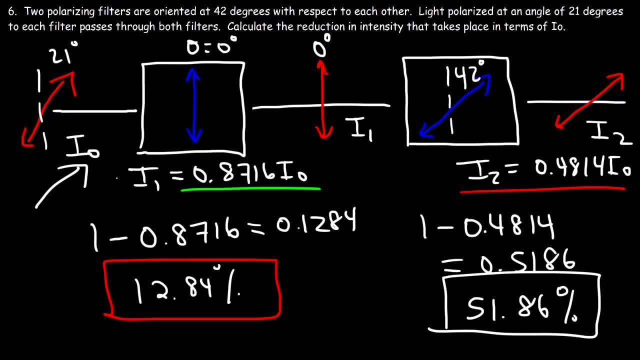 But we also need to do it in terms of I0.. So, in terms of I0, we could say that this reduced by negative 0.1284 I0.. And then, for the second one, we could say that it's negative 0.5186 I0.. 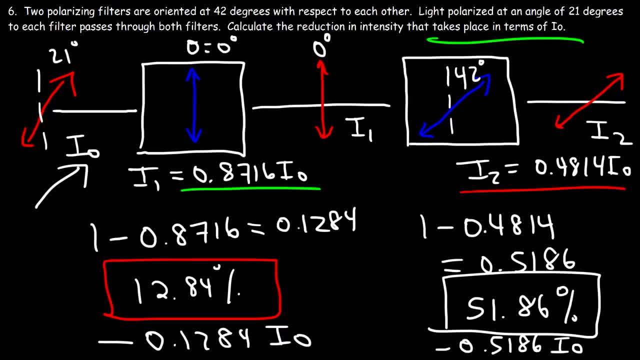 I almost forgot that We need to do it in terms of I0.. Now we should probably put a negative sign in front of the box. So we're going to put a negative sign in front of the box. So we're going to put a negative sign in front of the box. 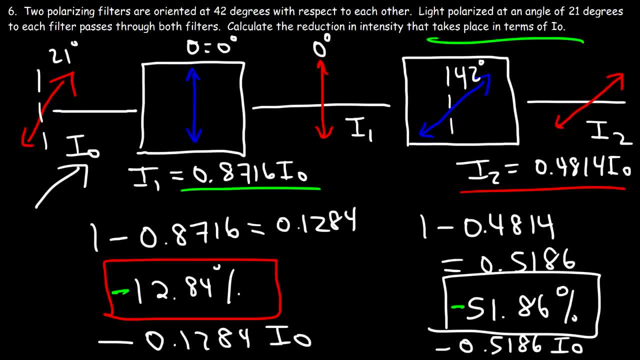 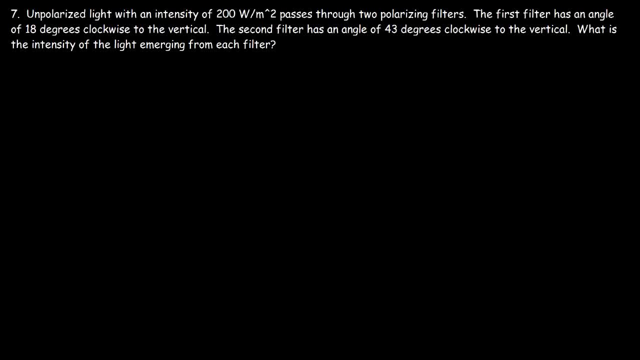 And now we need to do a comparison of the percentages. Or剛 넣ônmez sait unboxing остановmen prob. Let's rise to the next problem, Number 7.. Unpolarized light with an intensity of 200 watts per square meter passes through two. 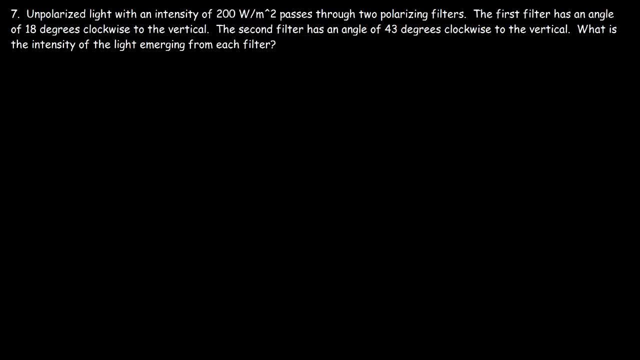 polarizing filters. The first filter has an angle of 18-degrees clockwise to the vertical. The second filter has an angle of 43-degrees clockwise to the vertical. what is the intensity of the light emerging from each filter? so we're 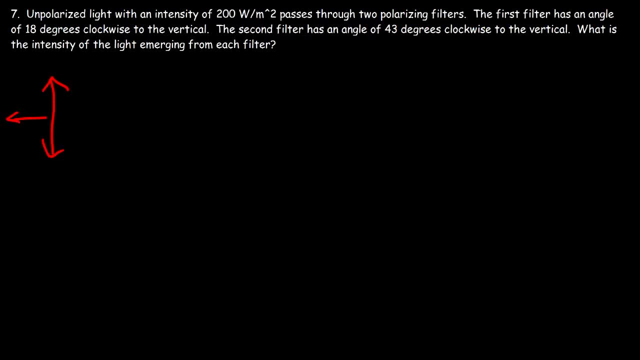 starting with unpolarized light, and it passes through two polarizing filters, the angle of which is specified. so the first one has an angle of 18 degrees clockwise to the vertical. so here's the vertical, and clockwise is flowing in this direction, in the direction of a clock. so we can say that this filter has 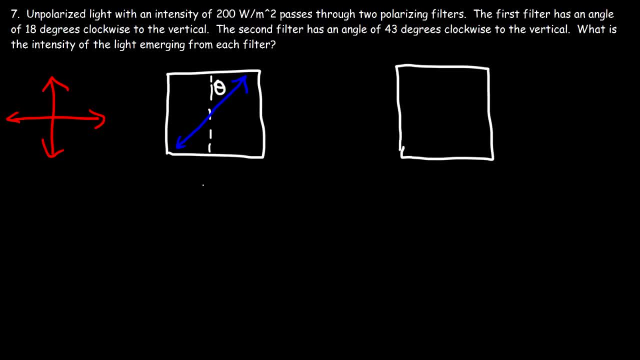 an axis that looks like this, where this is theta. so theta is 18 degrees from the vertical. now the second one is 43 degrees clockwise to the vertical. what is the intensity of the light emerging from each filter? so let's call this I 0, I 1 and I 2. so if we have unpolarized light becoming polarized, 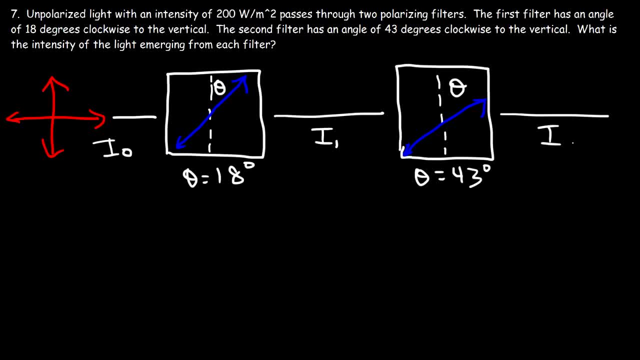 then it doesn't matter what the angle is. I 1 is going to be 1 half of the original intensity, so the light that passes through the first filter will be in the same direction as the first filter, that is, it's going to have an angle of 80 degrees relative to the vertical. now we 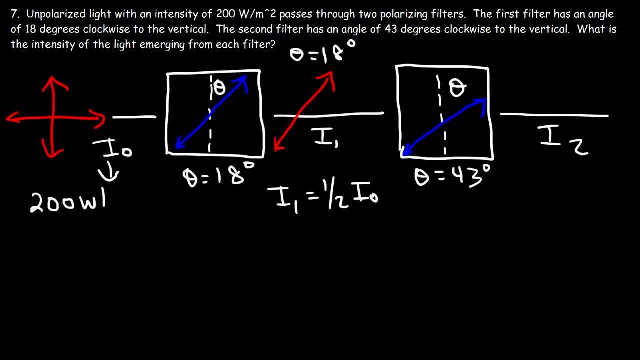 have the original intensity, its 200 watts per square meter. so I one has to be half of that. half of 200 is 100. so now we need to calculate I-2. so I 2 is going to be I1 times cosine squared of theta. You only should use this if you. 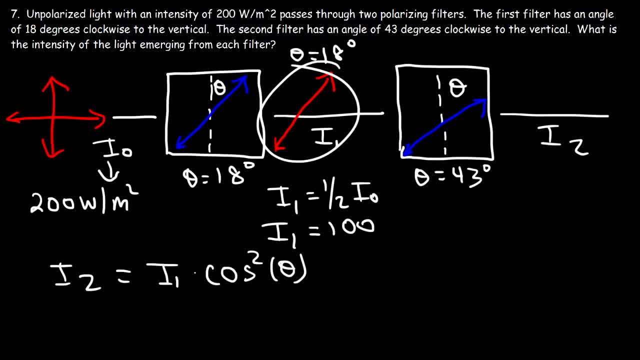 have plain polarized light or just polarized light in general passing through a filter. Don't use this equation if you have unpolarized light becoming polarized. It only works if you have polarized light passing through a filter. Now we know I1,, it's a hundred. What is the angle? So the angle that we 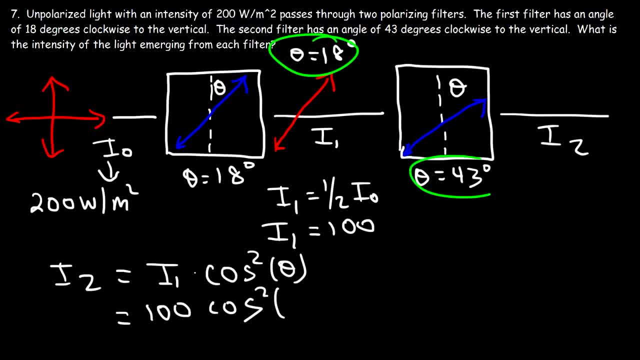 need is the difference between these two angles, The angle between the polarized light and the angle between the axis of the filter. So the difference in angles, that's 43 minus 18, so that's 25.. degrees, So it's going to be cosine 25 squared times 100.. And so the final 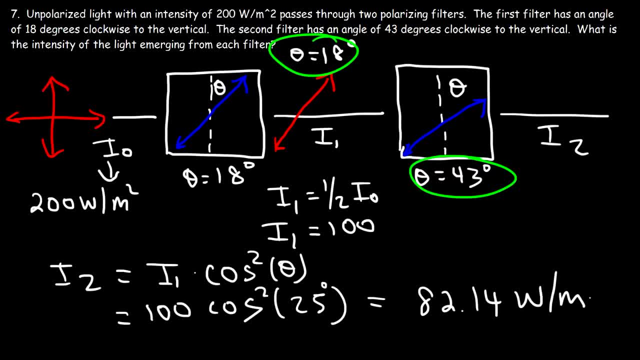 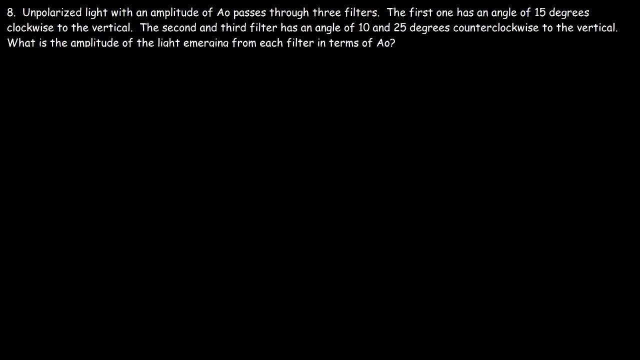 answer is 82.14 watts per square meter. So that is the intensity of the light that passes through the second filter, Number eight. unpolarized light with an amplitude of AO passes through three filters. So let's try this, Let's try the three filters. So this is filter number one, and then filter number two, and 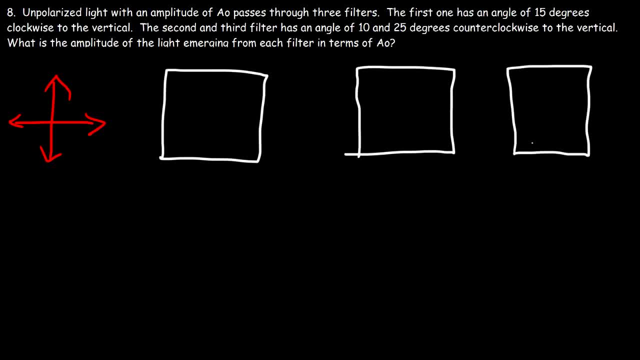 filter number three. Now, the first one, that is, the first filter, has an angle of 15 degrees clockwise to the vertical. So here's the vertical line and clockwise that's going that direction, in the direction of a clock, And so that angle is- I'm going to put it on top- 15 degrees. Now the second and third. 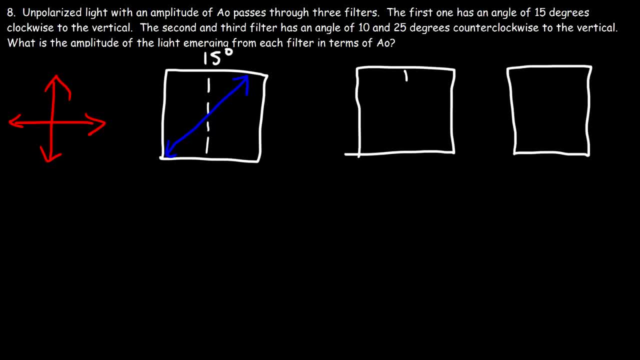 filter or the second one has an angle of 10 degrees counterclockwise, So we're going opposite from the direction of a clock. So this is going to be in this direction. So if we call this angle positive, I guess we can call the other one L. 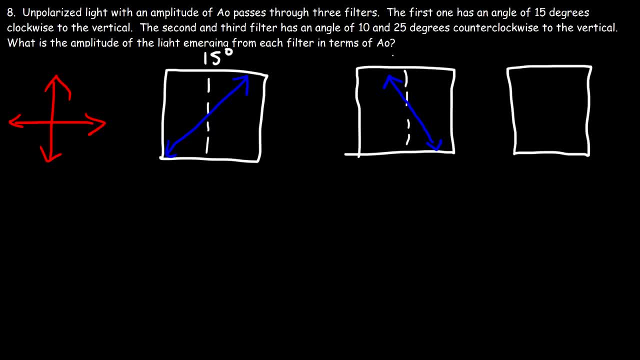 Now, technically, when you're dealing with most rotation problems, counterclockwise is usually defined to be positive and clockwise is usually defined to be negative. So just be aware of that. But for this particular example, since we've been accustomed to calling 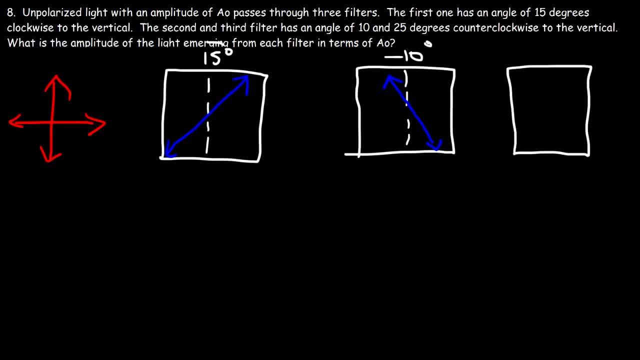 this angle aswer that we'll have to be careful, as weamatop. So to call this angle as a positive angle, we're going to make this one negative because it's going in the opposite direction, But you could change it up if you want to. The answer will. 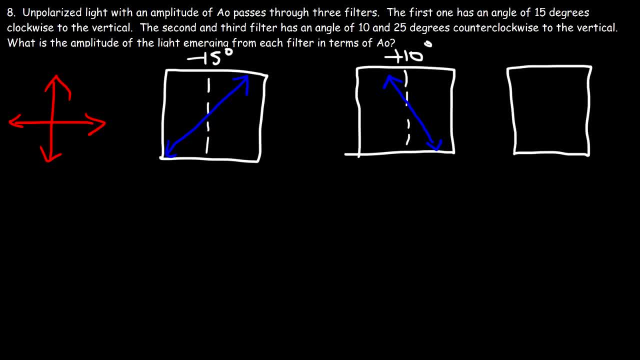 still be the same. If you make this negative 15 and this one positive, you'll still get the same answer. So just be aware of that fact. Now for the last one. it's 25 degrees counterclockwise, So let's bend it a little bit more. So I'm going to call this angle 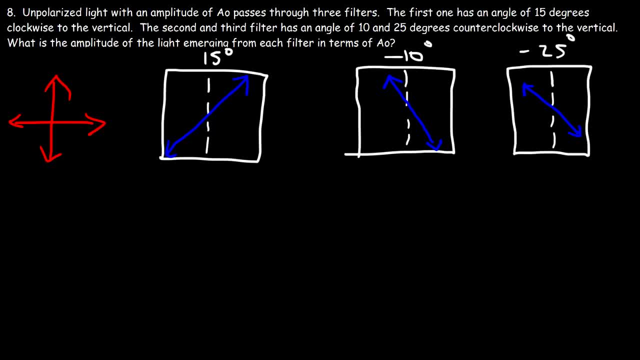 negative 25.. What is the amplitude of the light emerging from each filter in terms of AO? Now we need to know the relationship between amplitude and intensity. Intensity is proportional to the square of the amplitude, And you need to know this formula A is equal to. 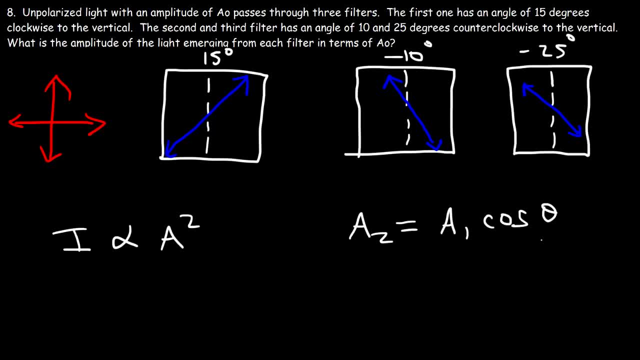 A, Let's say A2, is equal to A1 times cosine theta. Now if we square both sides of the equation we get: A2 squared is equal to A1 squared times cosine squared, And we can replace A squared with I. So this gives us Malice's Law for intensity as it passes through a filter. 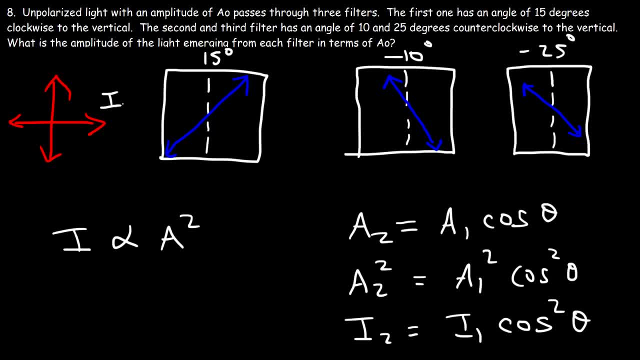 So keep that in mind. So let's say, if this was IO, then this would be 1.5 times cosine theta. So if this is AO, what should be A in this case? Well, this is going to be A1,, A2, and. 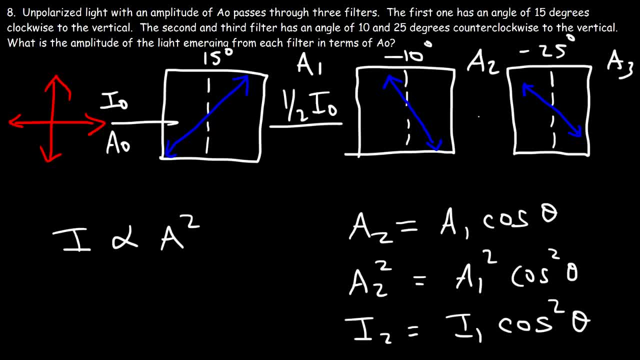 A3.. So what's A1 in terms of AO? Well, let's find out. If the intensity is proportional to the square of the amplitude, then we can say that the square root of the intensity is proportional to the amplitude itself. So we can write a ratio. 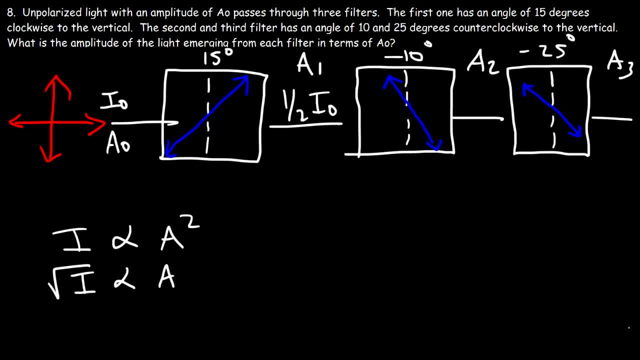 Of the intensities instead of equal to the ratio of the amplitudes. So we can say that A1 divided by A0 is equal to the square root of I1 over I0, because A is proportional to the square root of I. Now we know what I1 is in terms of I0. This here is I1.. I1 is: 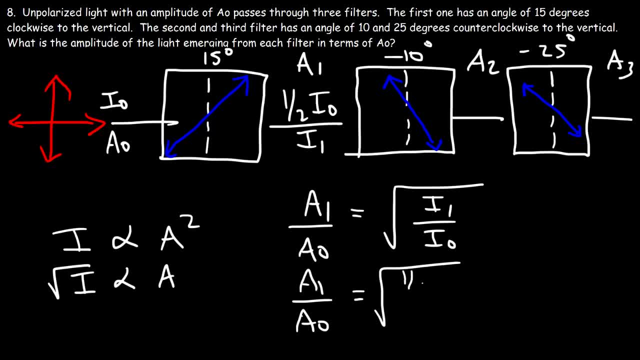 going to be half of I0. So let's replace I1 with 1 half of I0. So we can say that A1 is equal to the square root of I1 over I0.. We can see that I0 will cancel, And so A1 over. 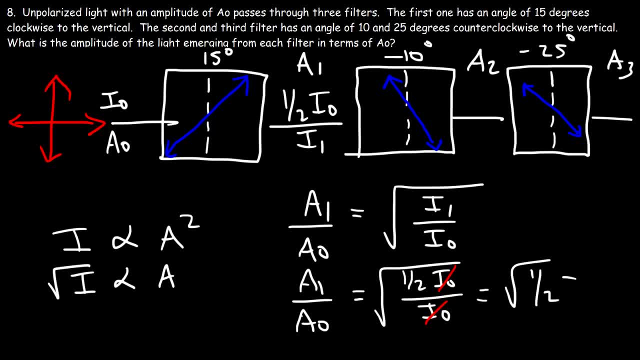 A0 is going to be the square root of a half. The square root of 1 is 1 and the square root of 2 is itself. So let's multiply the top and bottom by the square root of 2.. And so we can see that A1 divided by A0 is equal to the square root of 2 divided by 2.. These two, when multiplied, you get the square root of 4, and the square root of 4 is equal to the square root of 2 divided by 2.. These two, when multiplied, you get the square root of 4, and the square root of 4 is equal to the square root of 2 divided by 2.. These two, when 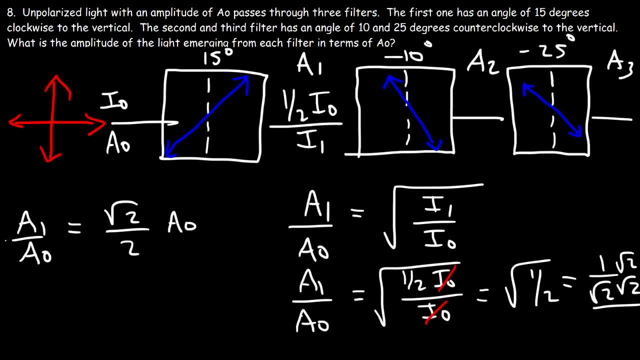 4 is 2, and so if we multiply both sides by a 0, we can see that a 1 is equal to the square root of 2 over 2 of a 0. that took a while. hopefully you followed what we just did, so let's write this answer here and now. let's move on to the second. 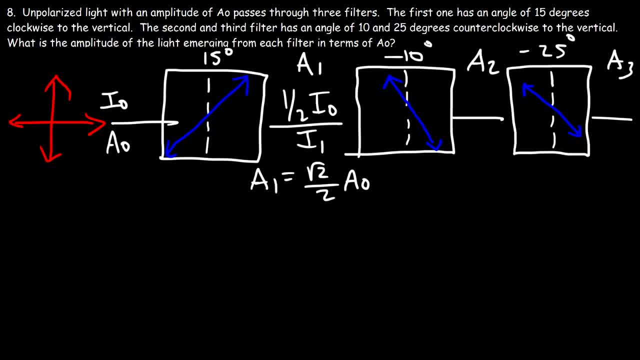 part of the problem. so now the light that passes through the first filter will be in the same direction as the first filter, and then through the second one, it's going to be parallel to it, and then the third one is also going to be parallel to the third filter. so now the angle difference between the filter and 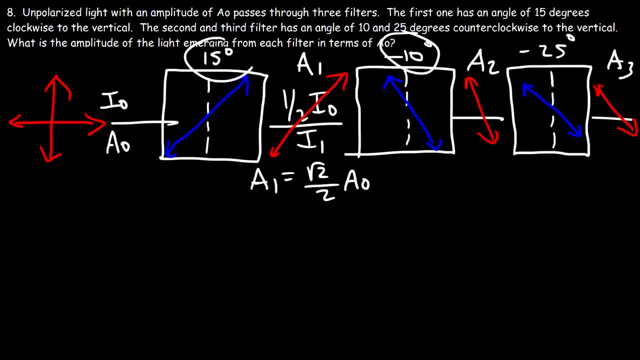 the light is basically the difference between these two filters and that's why I wanted to assign the angle difference between the filter and the light to the light. so I'm going to assign this value as negative 10 instead of 10, because if you subtract 15 by 10 you get 5, but if you subtract 15 by negative 10, that will. 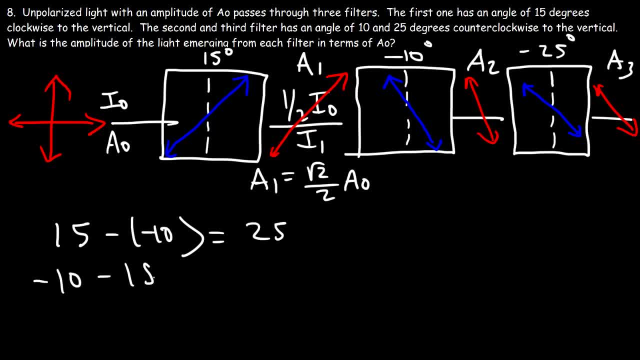 give you positive 25 or if you do negative 10 minus 15, that's negative 25. cosine 25 and cosine negative 25 is the same plus when you square it it's automatically going to be positive. so the order in which you subtract it will. 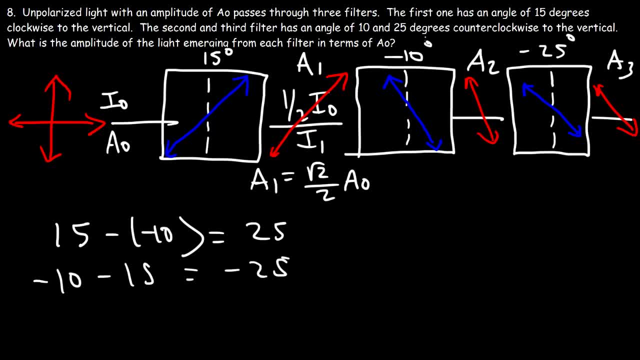 not affect your answer. However, you do want to make this negative 10, because you don't want to get a difference of 5,, you want to get a difference of 25, and that will affect your answer. So the relation between a2 and a1 is as follows: a2 is a1 times cosine theta and it's not squared. 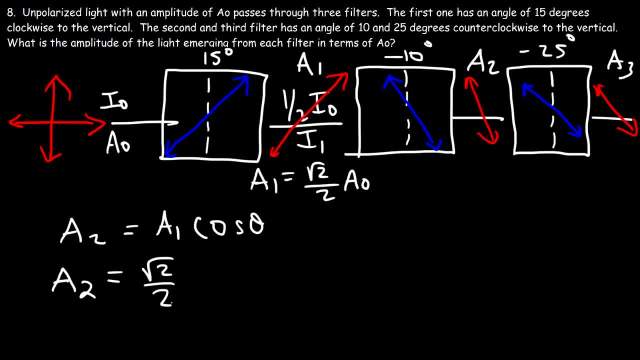 So a2 will equal a1, which is the square root of 2 over 2 times a0, times cosine of 25.. Now, cosine 25 is not a nice number, so we'll need to report it as a decimal. Cosine 25 is 0.9063, and if you multiply that by the square root of 2 over 2, then you should. 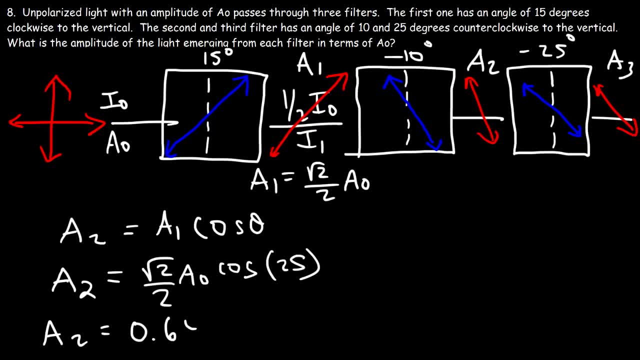 get a2 as being 0.6423.. Okay, 0.9 relative to a0.. So now let's move on to a3.. So a3 will be equal to a2 times cosine theta, And so this angle here is the difference between the angles of the two filters. 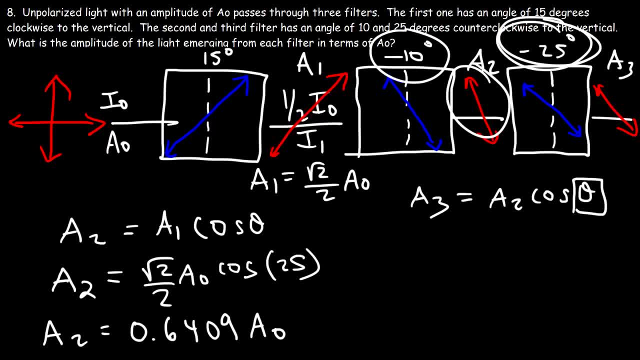 Or you could say the angle of the filter and the angle of the light, that the polarized light that passes through the third filter, which would be the same as that angle, so it doesn't matter. Now, the difference between negative 25 and negative 10 is negative 15.. 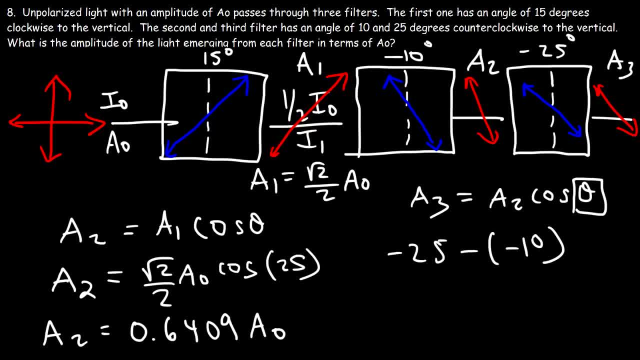 So if you take negative 25 and subtract it by negative 10, or if you do it in the other way, it doesn't matter. In this case this will give you negative 15.. If you do it in the other way, it's going to be positive 15.. 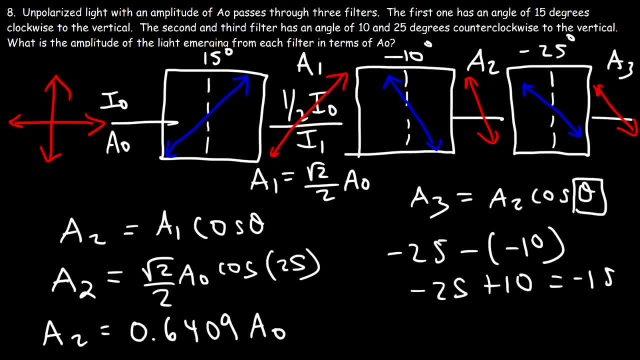 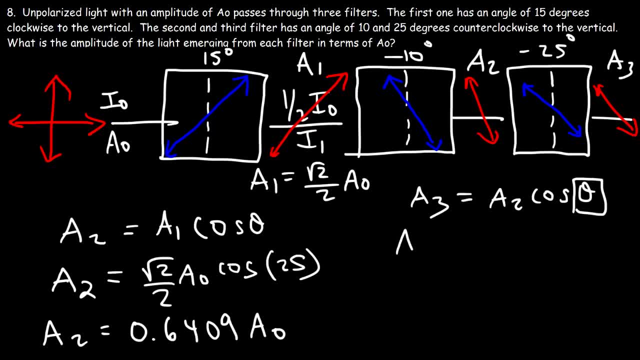 So a2 is a2.. So a2 is a2.. So a2 is a2.. So a3 is going to equal a2, which is this thing right here. So that's 0.6409 a0 times cosine of 15 degrees. 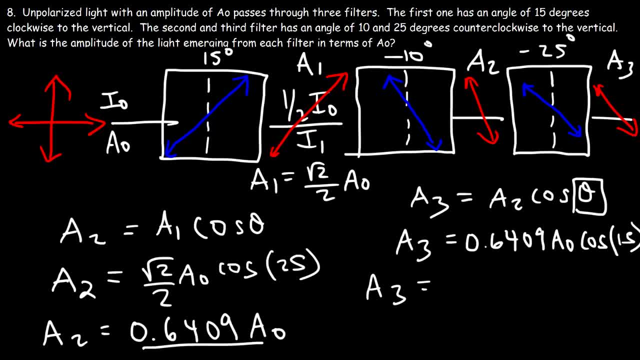 Now, cosine 15 is 0.9659.. If we multiply that by 0.6409.. Oh, you can see that a3 is 0.619 of a0. so these are the answers: this one, this one and this one. 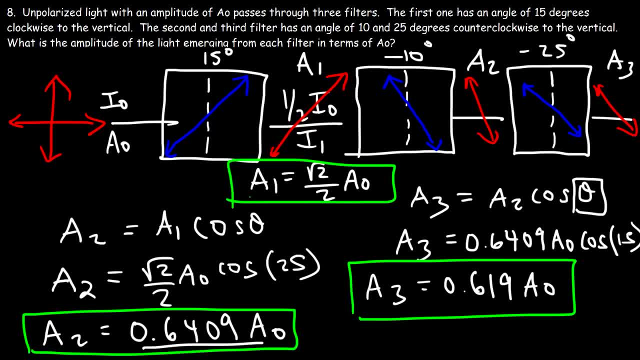 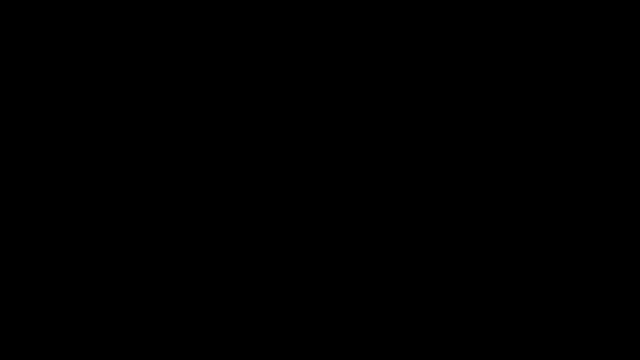 so that's the amplitude of the light emerging from each filter in terms of a0. so